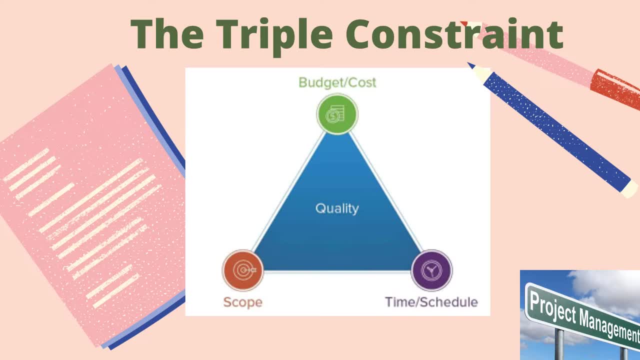 manager or as part of the project team, you might encounter circumstances or situations wherein you have to modify things, And when you modify things, sometimes it's going to affect other variables as well. So, taking a look at this triple constraint- scope, time and budget- once you touch one of these variables, it can potentially affect. 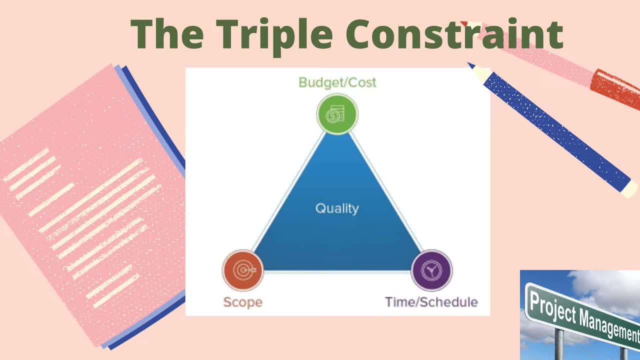 the other variables, including quality, Scope, time and budget, are variables greatly affecting quality. With bigger scope, quality might be missed, especially if we work on a smaller budget and a tighter schedule. Now what if we reduce the cost? What's going to be the effect of that to your scope, to your ability to create? 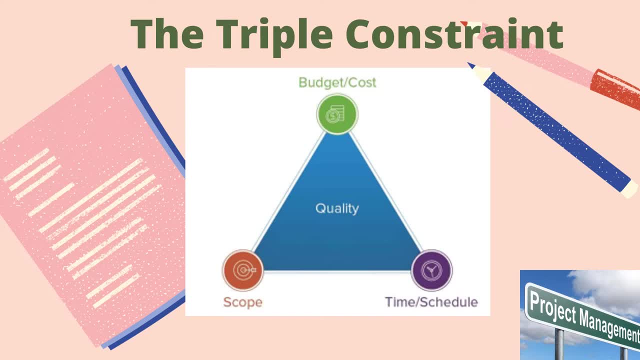 that project and to the quality of the project and, at the same time, to your, to the probability of delivering the project on time. Say, for example, I will ask you in my class to create minute video as a project that will be submitted next week. given that time and 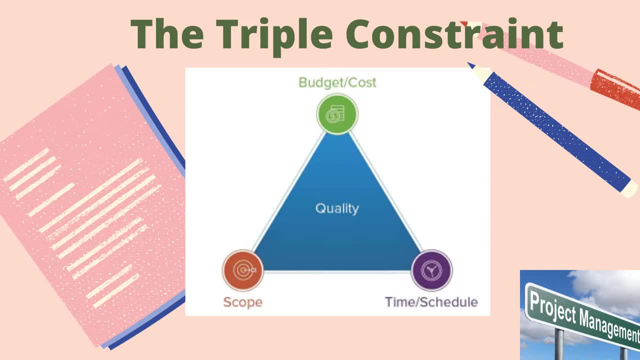 given the scope of this activity, you might be able to do it easily because of the scope, which is smaller, and the time, which is quite enough for you to build or to create a video. but what if I change my mind? what if I say: okay, instead of a one-minute video, submit a 30-minute video, to be submitted next. 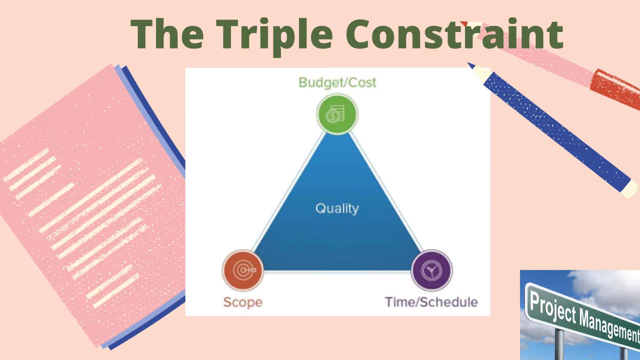 week will it change some things. will it change the quality of your output? will it affect your ability to produce the video on time? will it be able to change the budget for the video? what if I don't change the scope? what if I say, okay, so let's stick with a one-minute video, but you have to submit it in two days? 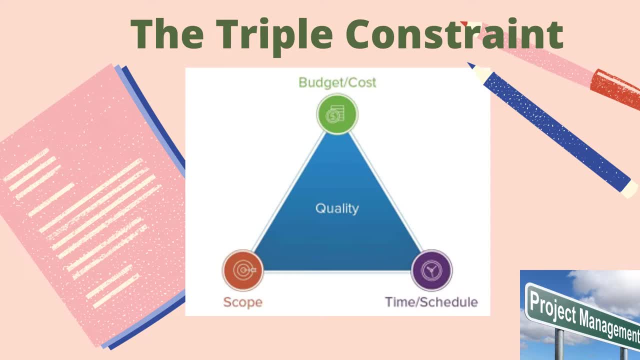 okay. will still it affect quality or the cost or the scope of your project? the answer is usually yes, and you can see there the interdependence or the relationship that is existing among the three variables, or the triple constraint, in this particular situation. so why are we trying to understand this as managers? 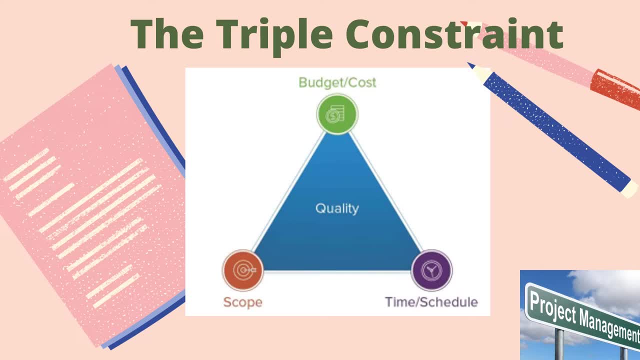 we need to understand this, because you will be making decisions, or you will be making decisions later on that might have effects on one of those things mentioned now. why do you have to make decisions later on? I'm not telling you to really do it, but you, you cannot avoid certain risk or certain modifications. 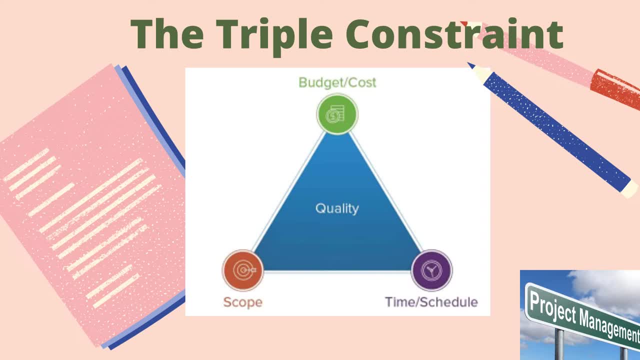 especially when one of the things that you cannot control happen to change and you don't have a choice but to go with with those changes. so when you do that, you might compromise your or you might change your scope, you might change your budget, you might change the time and potentially it can change the quality. 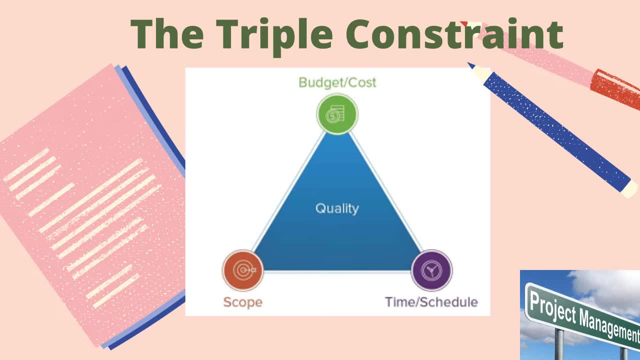 so, basically, the triple constraint is telling us that there will be a trade-off. when one of these things and one of those variables change, your job is a project manager to balance those changes. there will be a trade-off. there might be losses, there might be sacrifices. so it is. 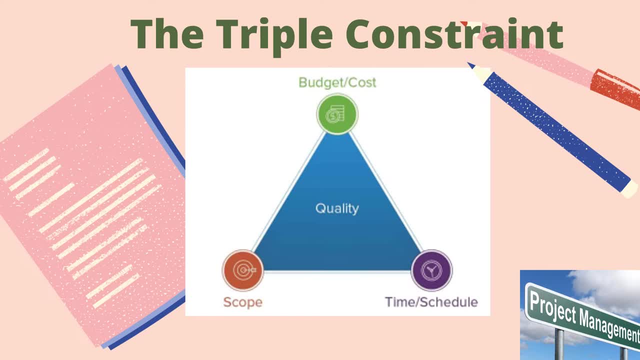 your past to minimize the sacrifices and minimize the losses, because you have to go back to your project acceptance criteria. so what if your objective this? would you give up your objective just because your budget has decreased? if you do that, then you are not really managing the project because you just 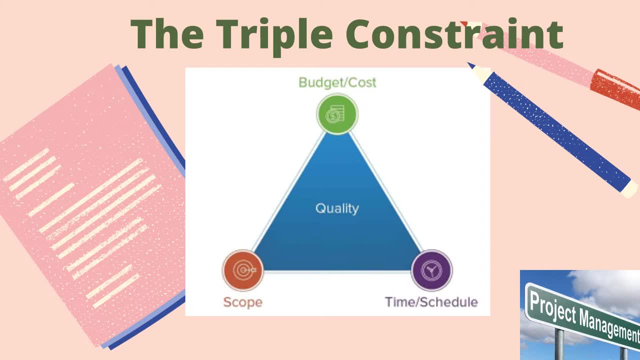 don't give up on it. you have to find ways to be able to carry it on. so I hope that later on, when you do your project, when you do these things and you experience certain changes, you go back to the triple constraint and you try to analyze what's going to be the consequence, if ever one of those things. 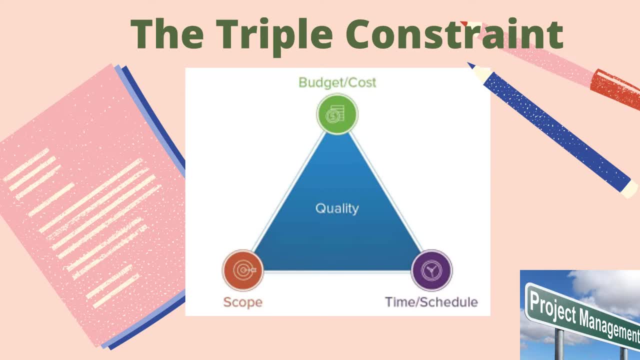 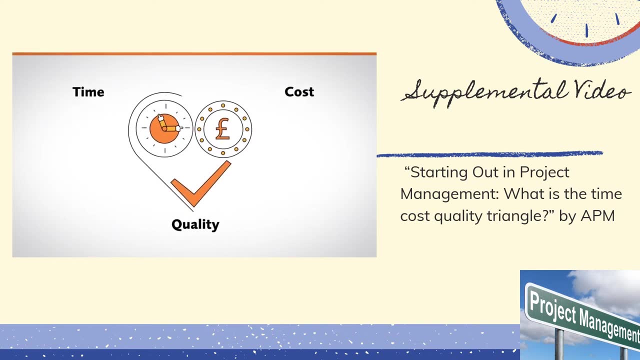 will be changed. time, cost and quality are at the heart of project management. for example, the project must be completed by a specific date. the project must be completed by a specific date, the project must not spend more than the agreed budget and the products and services created must meet a defined specification. but because projects are 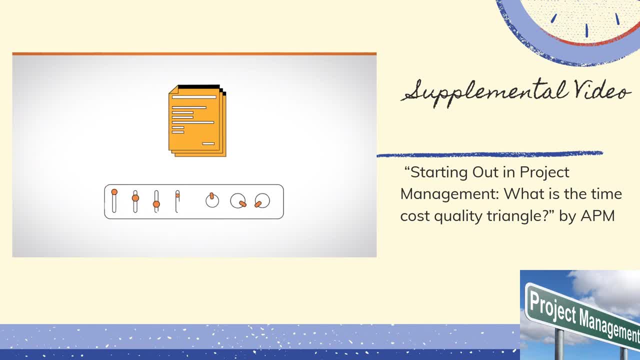 unique and we don't know exactly what will happen. there's a good chance that you'll need to adjust the balance between these parameters over time. this means a trade-off: to take more time, spend more money or agree to reduce the scope and all the quality specification, for example, if you're delivering a new 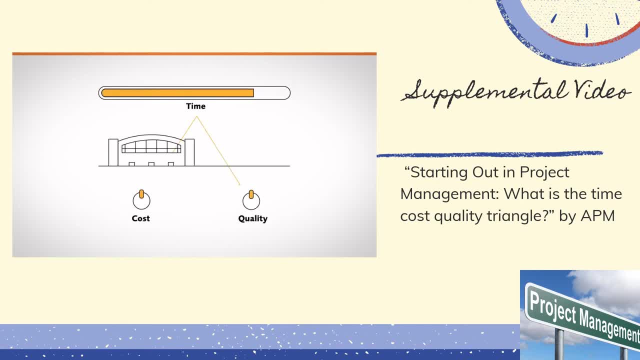 sporting facility to a deadline for a major competition, then you would choose to either spend more money and or reduce specification in order to meet the date. if the date wasn't critical, you may choose not to trade scope for time and take the time and spend the money you. 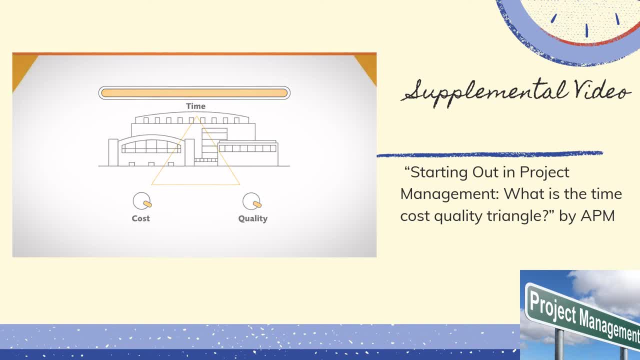 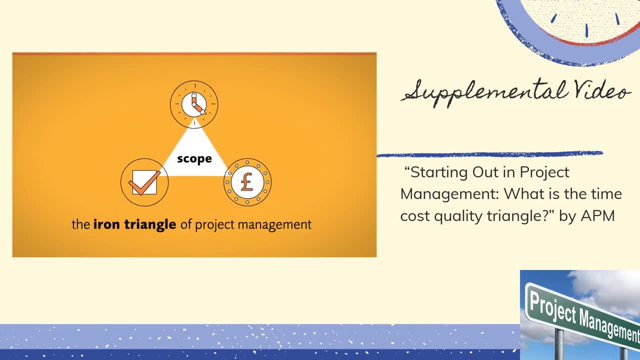 need to get the product you designed. the three parameters of time, cost and quality are often referred to as the iron triangle of project management. balancing the three is sometimes called the project managers trilemma. the trick is to understand the relative priority of objectives and the cost of the project. 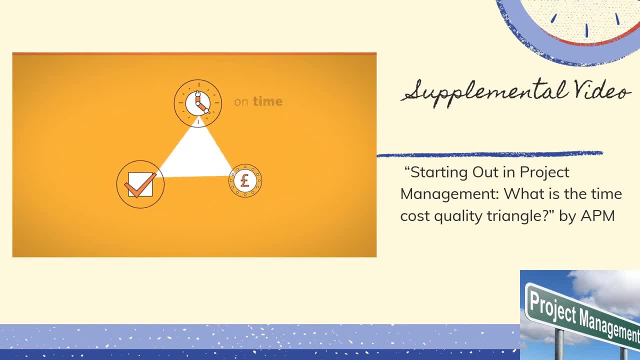 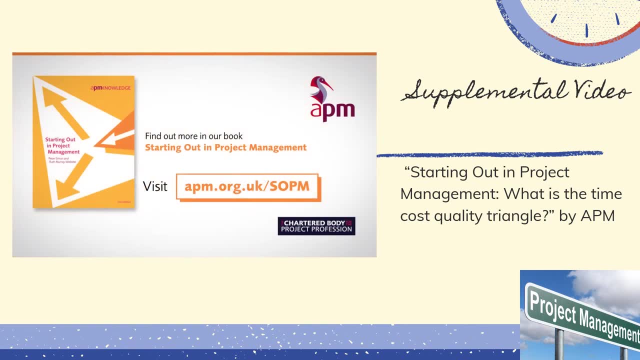 is it more important to finish on time, on budget or to the right quality to keep the customer or sponsor happy? you can find out more about the triangle and other project management fundamentals in our book starting out in project management: visit APMorguksopm. now. notice that there is a little bit of. 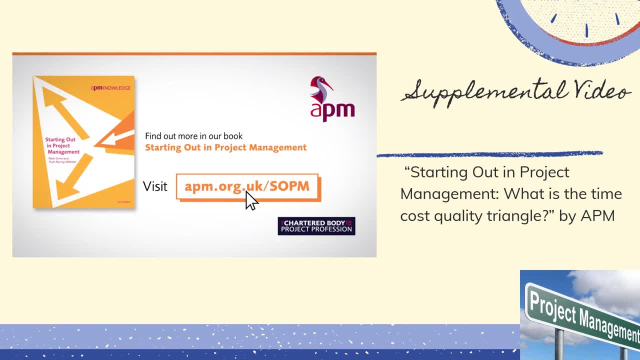 difference in our discussion because in their triple constraint they have included quality as part of the three main variables, while scope is in the middle. in my case, I have included scope in the three triple constraint and the quality is in the middle, you know, being the the variable. 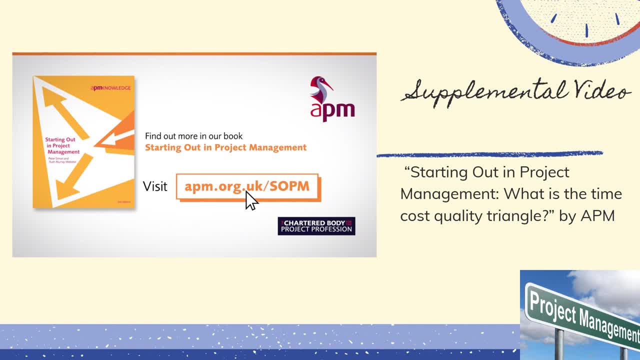 that will be affected by any of those changes in your scope, time and budget. but as you listen also to the discussion, you will also see the similarity in my discussion and a discussion in the video. bottom line is it is simply telling us that when one of those variables change there.